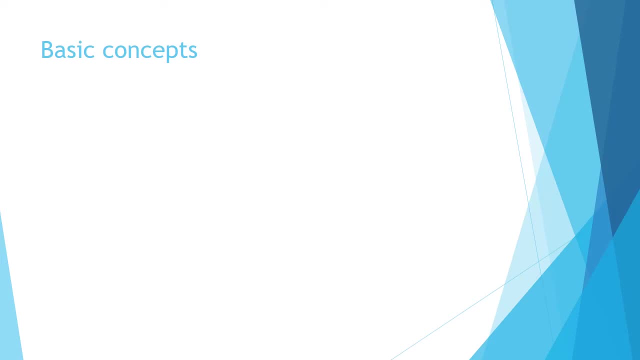 why is it important? we're saying all those things are the basic concepts of economics. First, let's look at the definition It's saying: economics is the study of how individuals, businesses, governments and other organizations within our society chooses to use scarce resources to satisfy their unlimited needs and wants. 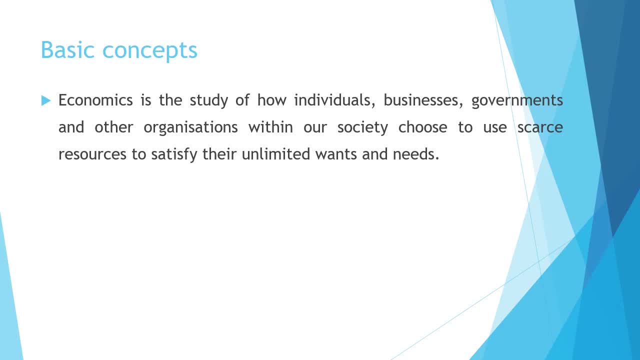 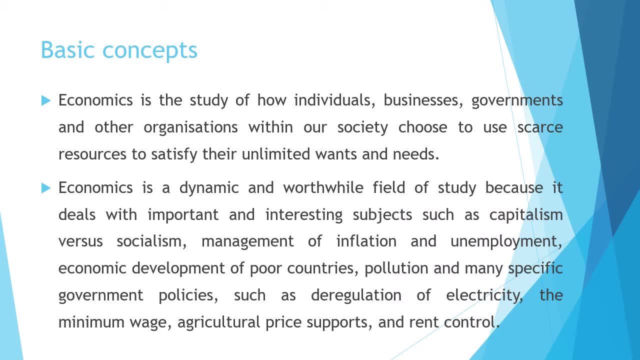 So you might ask yourself: why is it important for me to know this subject? Here's your answer. It is important for one to study economics because it studies, or it deals with, important and interesting subjects such as capitalism versus socialism, management of inflation and unemployment. economic 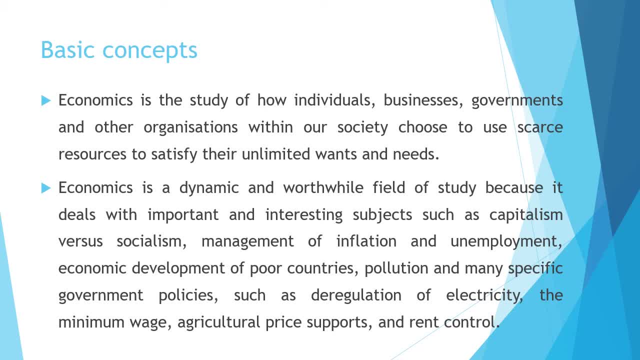 development of poor countries, pollution and many specific government policies, such as the regulation of electricity, the minimum wage, cultural price supports, as well as rent control. So basically, we're saying that economics it has to do with our daily lives, what is happening to us every day, So that is what it does. 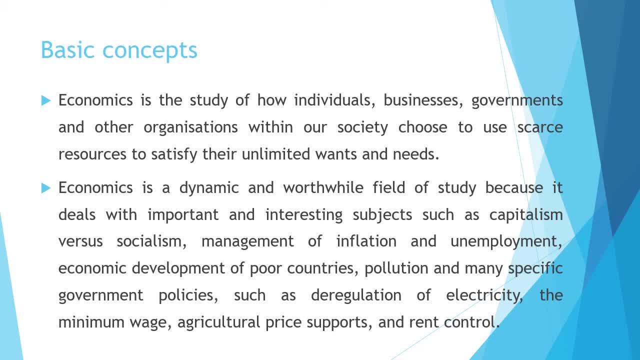 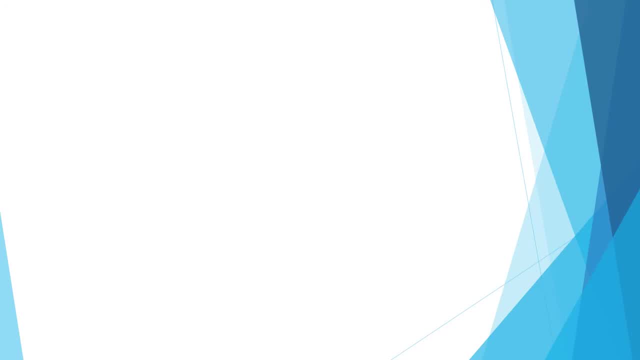 it just focuses on the things that we see every day, things that takes place in our lives every day. So we're saying that in economics we have limited resources and unlimited needs and wants. So when we study economics, economics tells us that resources are limited, so we need to know how to work. 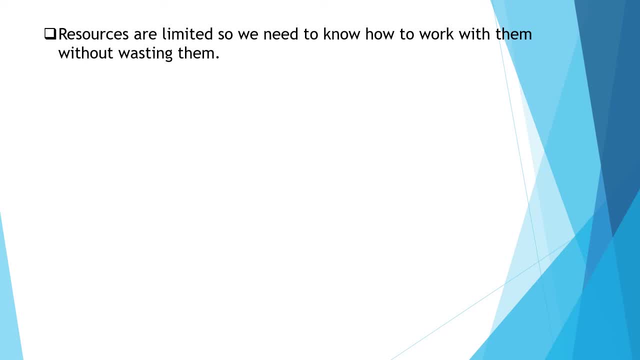 with them without wasting them. So this is what you should put in your mind. Okay, fine, When I learn the subject economics, I will know that resources are limited, so I must find a way of using them without wasting them. And then the other point is because we cannot certify all our needs and 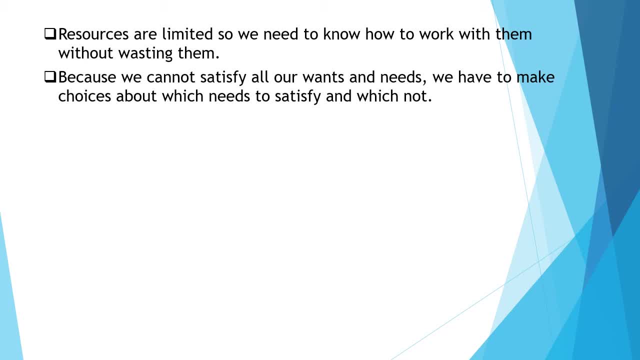 wants. we have to make choices about which needs to satisfy and which not. Remember, as individuals or as human, we're having unlimited needs and wants, or else they are limited resources. So whenever we have to use those limited resources- which means we have to choose- make a choice of which other needs and 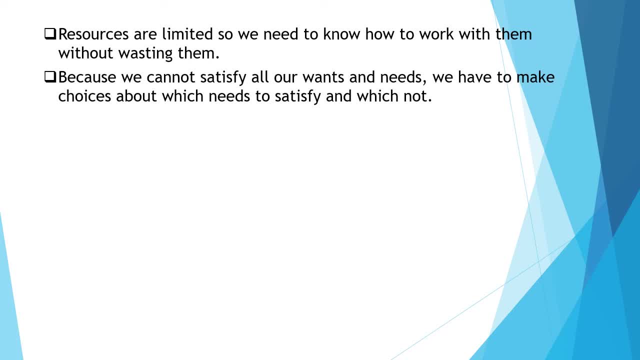 ones are we going to forgot and then which other ones are we going to certify? so economics allows us to make those decisions and that may lead to what we call the economic problem. how do we face economic problem? that's the question one may ask him or herself. okay, i know that i have limited 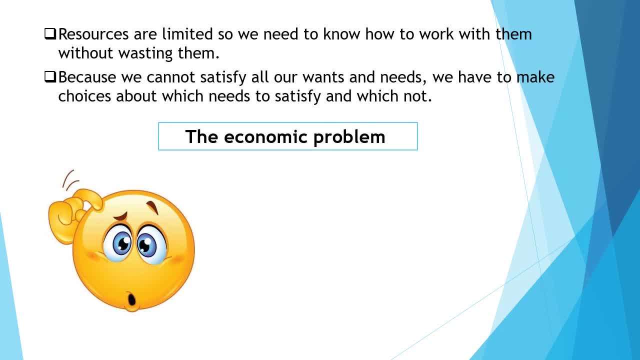 resources. and what's the problem? because i will choose which needs anyone to satisfy. but remember that will lead to what we call the economic problem. first we're saying the basic economic problem is scarcity. the problem arises because resources are scarce, but economic resources are better than the basic economic problems we want to address. 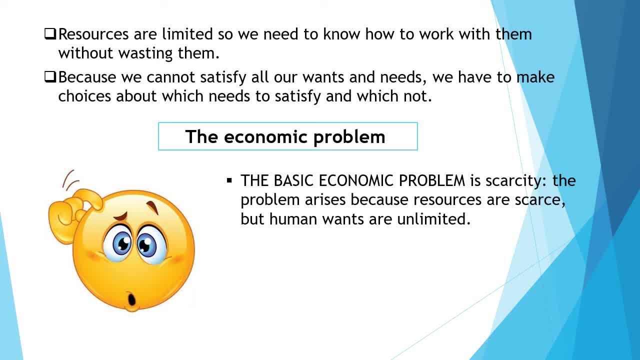 human ones are unlimited. we have those limited resources, which are also scarce to find. but as human we keep on wanting more and more and more and more of things. so that leads us to the problem of scarcity. for example, let's say you are in a class, in a class of 50 learners or 40? let's just say 40 and you know. 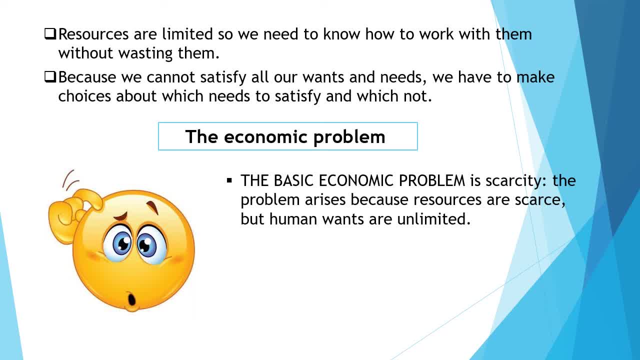 class and when you are 40, the class only have 30 chairs, which means we can say that the class has a scarcity of chairs because we are 40 and there are only 30 chairs, which means 10 people will not have chairs, so we have a 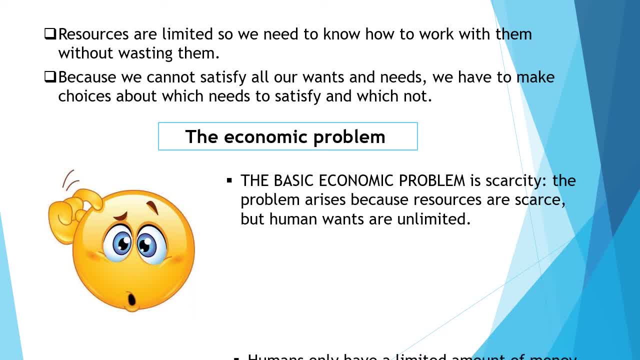 scarcity of chairs in the class too, and the other one was saying: human only have a limited amount of man, yet they have lot of needs and wants to satisfy. it may happen that I'm only having 1000 rand in my pocket, but I have lot of things that I want to. 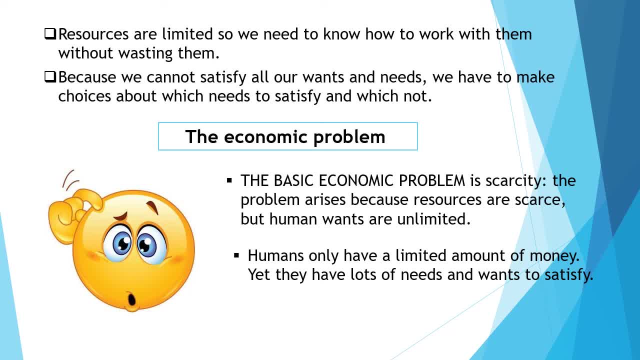 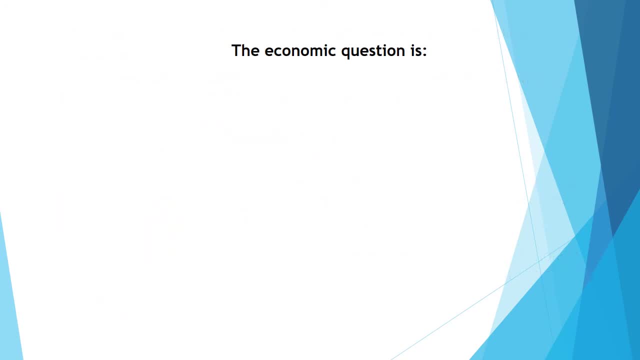 buy with that thousand and when I calculate those things they are more than the thousand itself. so you can see I have a limited amount but I have a lot of needs and wants to satisfy the economic problem that we have. it now leads us to what we call the economic